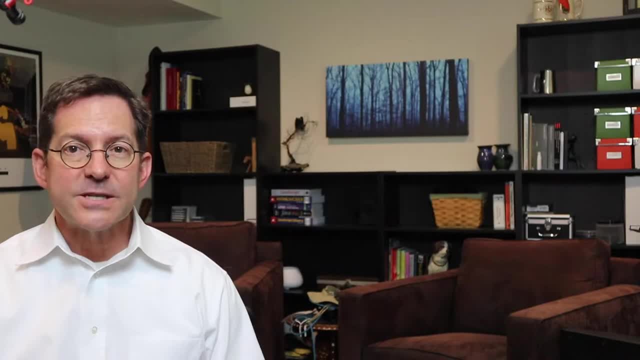 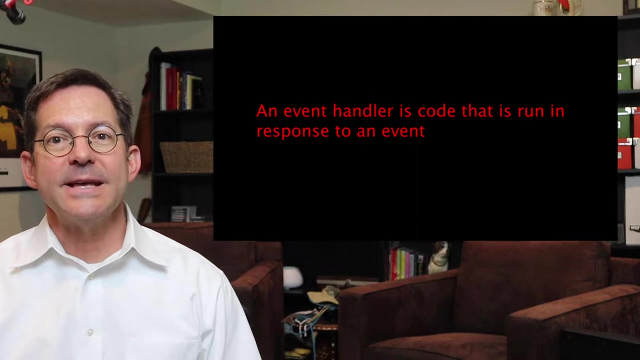 Events occur all the time in the browser. It's the programmer's job to determine which events should have actions attached and which events should not. If a programmer decides that an action should happen, code will need to be written. An event handler is the code that runs in response to an event. 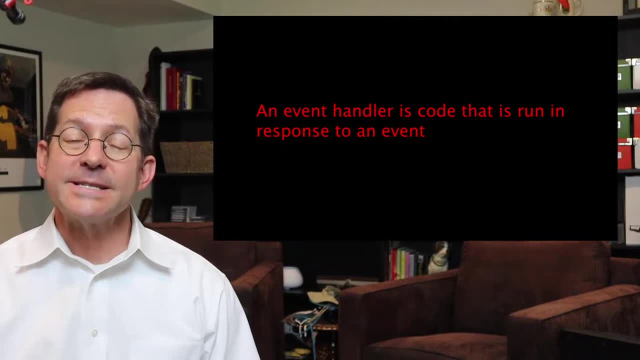 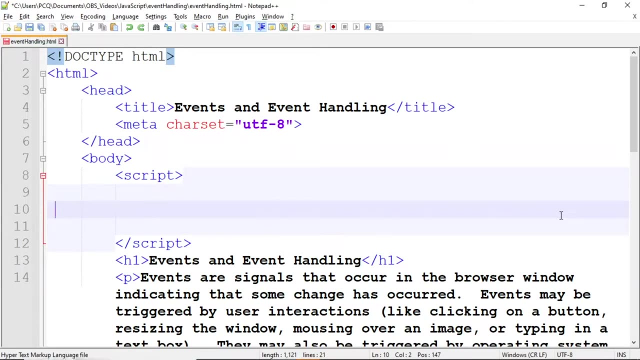 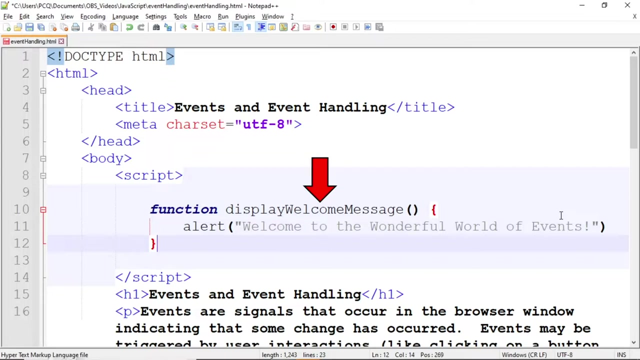 To better understand events and event handlers. let's take a look at an example. I've opened an HTML template and inside of the script tags I'm going to add a function. This function is called displayWelcomeMessage. You'll notice the function takes no parameters. 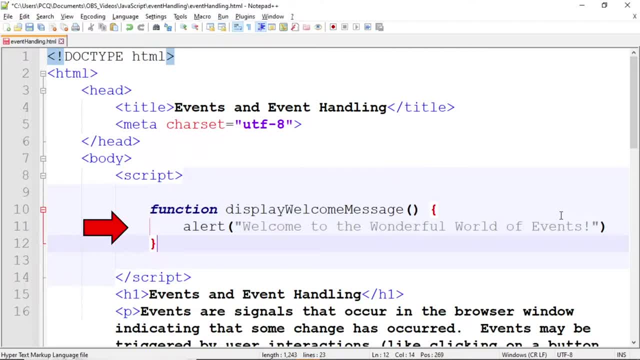 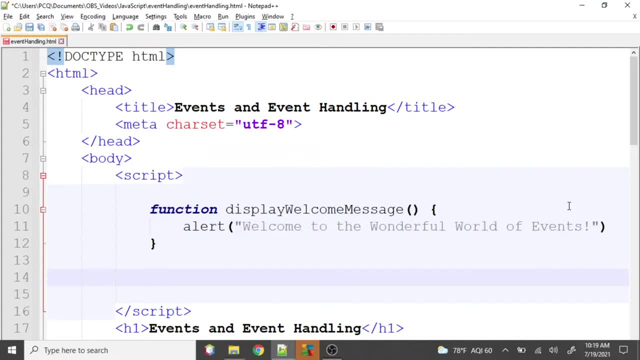 and does nothing more than display an alert box with the words Welcome to the wonderful world of events, The function name, followed by any arguments. However, I want this function to run when all of the contents for this web page load, I'll add window onLoad. 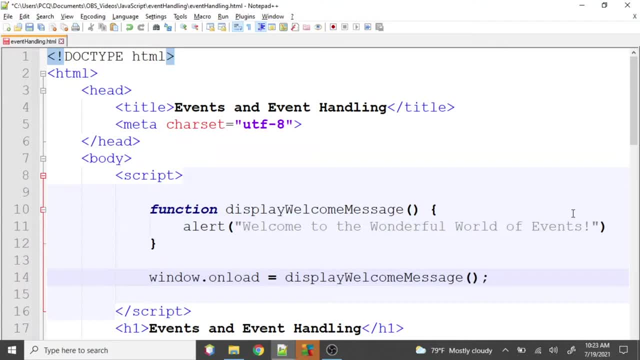 and assign it to the function call. The window object refers to the browser window that we have open. This object has an event property called onLoad. The onLoad event fires when the HTML document and all of its contents load. This additional content can be any scripts, images, stylesheet, references and so on. 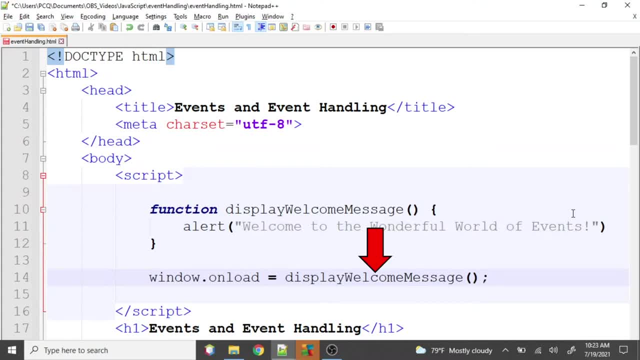 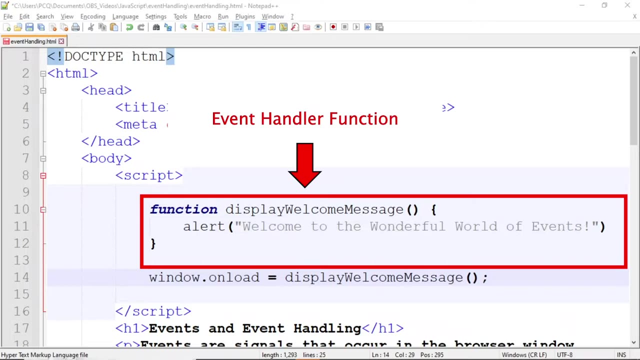 We assign the event the function that we want to execute when the event occurs. It's important to point out that this method of calling a function when an event occurs has two parts. First, there is the event handler function. This is the code that we wish to execute when the event occurs. 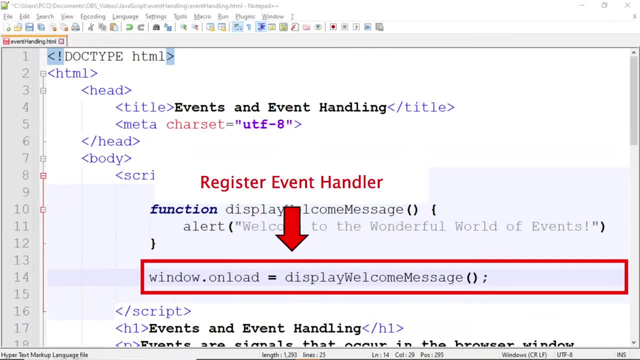 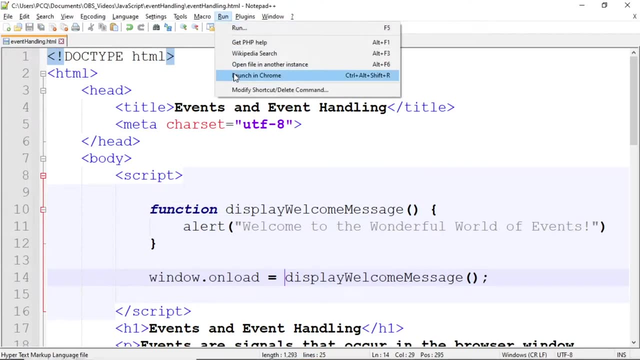 Second, there is the statement that registers the event handler function. This statement includes the object and the event, along with any assignments to our event handler function. We can save and run our code and you'll notice when the window onLoad event occurs. 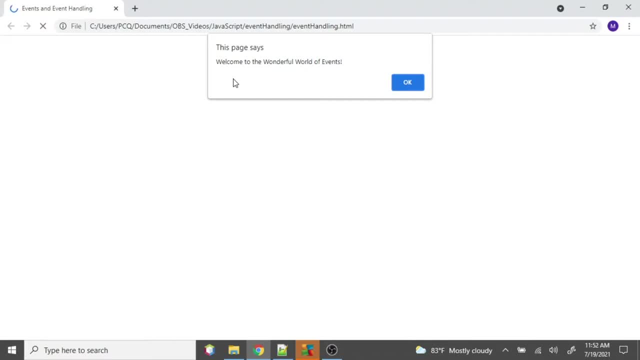 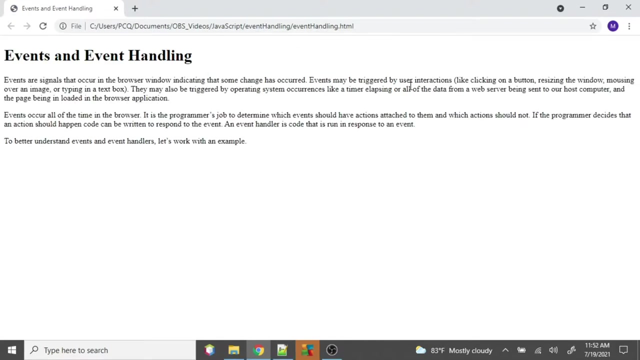 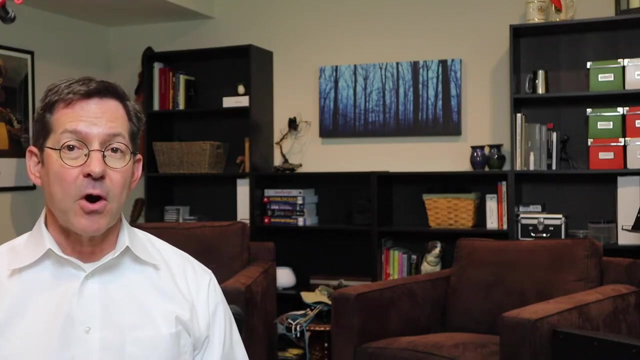 the display welcome message function is called and the alert box appears. It's important to recognize that the window onLoad event occurs before any HTML text is displayed. When I click the OK button, the text from the HTML body appears. Now that we know how to trigger our event handler function. 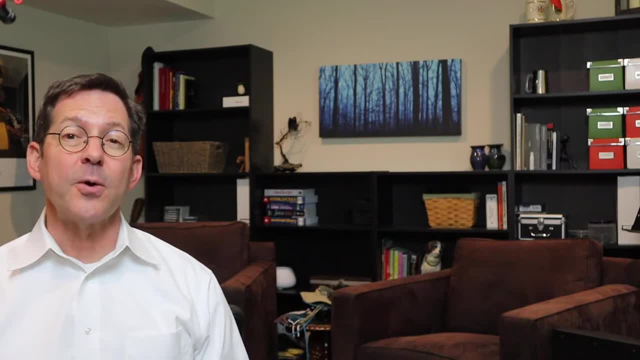 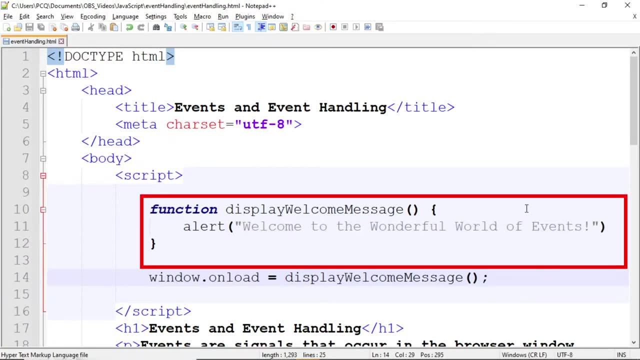 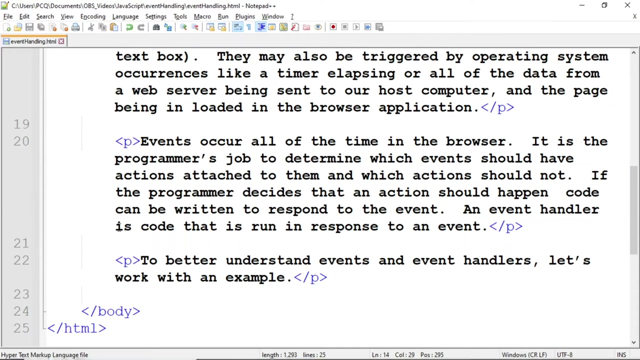 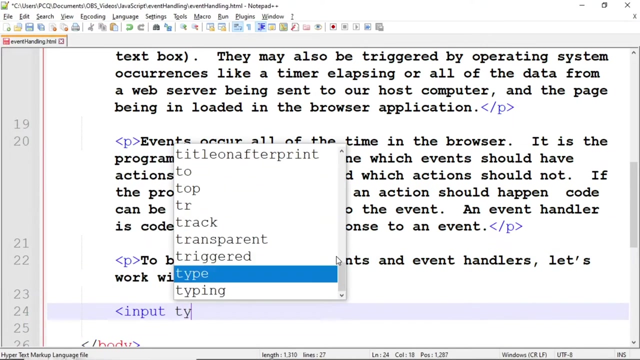 let's run our code. when a user clicks on a button For this example, we'll use the event handling code that we created in our previous example. when demonstrating the window onLoad event, We'll start by scrolling down and adding an HTML button. I'll type input: type equals button. 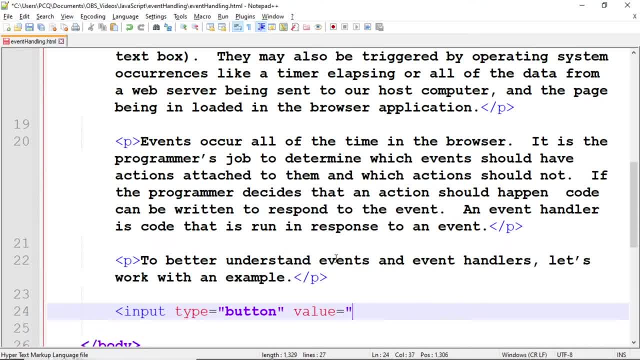 Then I'll. type: value equals welcome. The input tag allows me to create different types of input objects in HTML. I can create buttons, drop-down boxes, text boxes and so on. Here I want to create a button, so I use the type attribute and assign it to button. 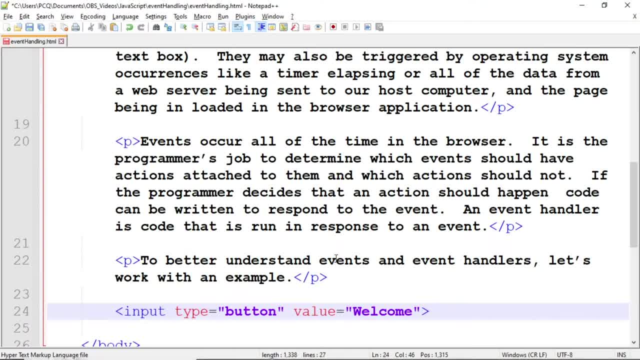 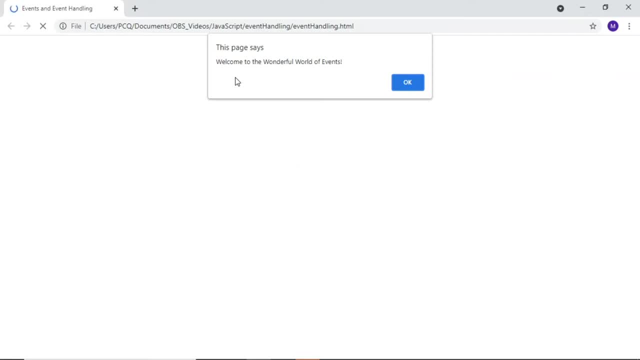 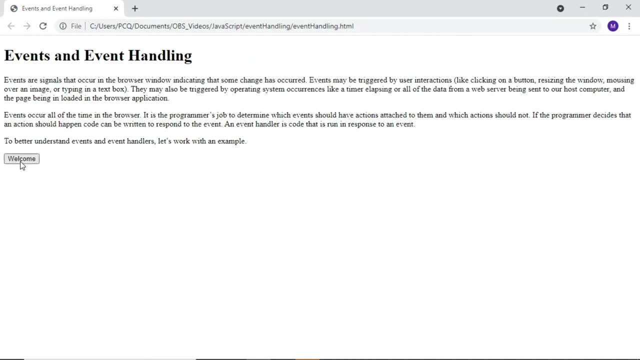 I want the word welcome to appear on the button, so for value, I assign it the string welcome. I'll save my work and display it in the browser. After clearing the alert box that displays for the window onLoad event, you'll notice that a button appears on my HTML page. 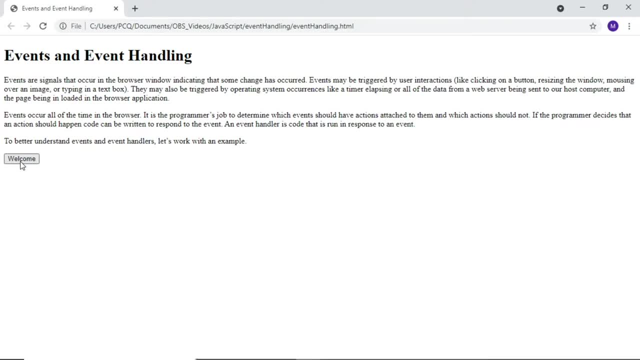 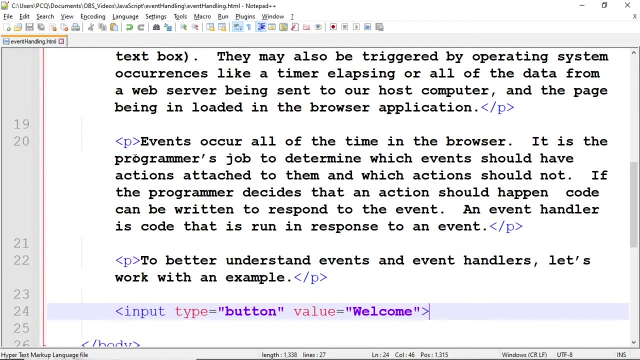 Although the button exists, you'll notice when I click on the button it does nothing To make the button functional. we need to register our JavaScript function by adding the onClick event to the button. I'll type onClick as the event. Next I'll type the assignment operator.